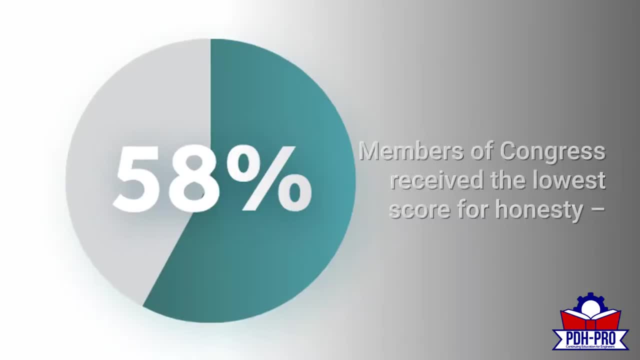 pharmacists, etc. – was ranked second overall. This is because engineers were ranked fifth overall and the medical profession – nurses, doctors, pharmacists, etc. – was ranked fifth overall took the other top positions. Members of Congress received the lowest score for honesty. 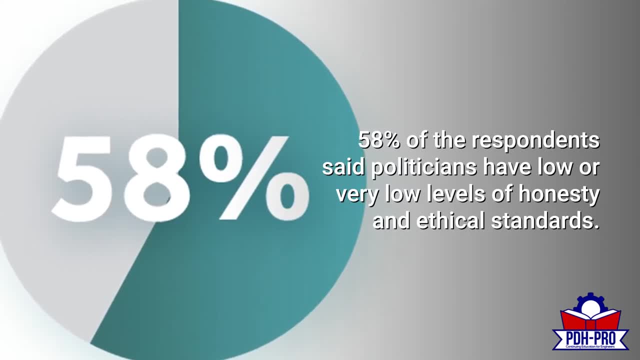 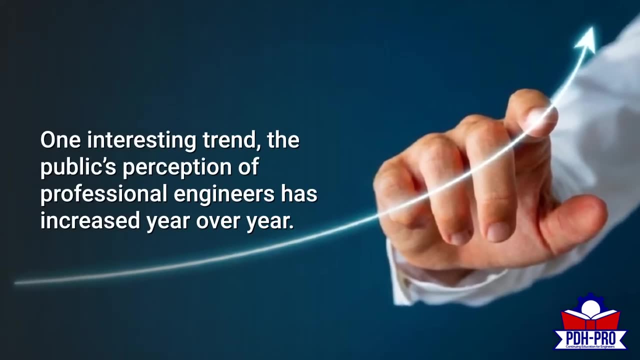 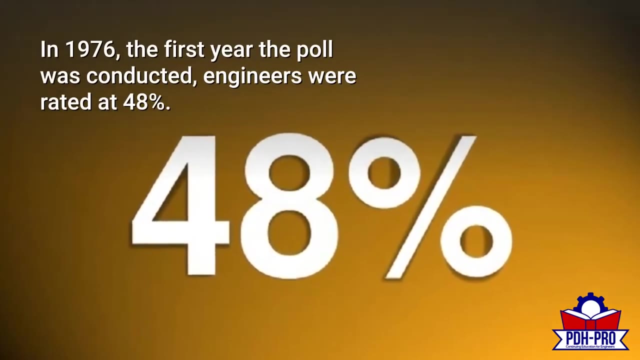 Fifty-eight percent of the respondents said politicians have low or very low levels of honesty and ethical standards. One interesting trend – the public's perception of professional engineers – has increased year over year. In 1976, the first year the poll was conducted, engineers were rated at 48% By 2016,. 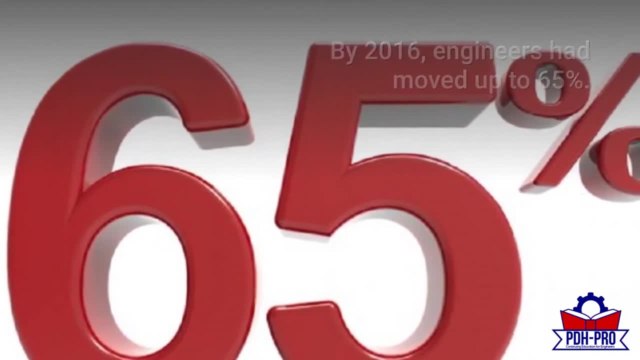 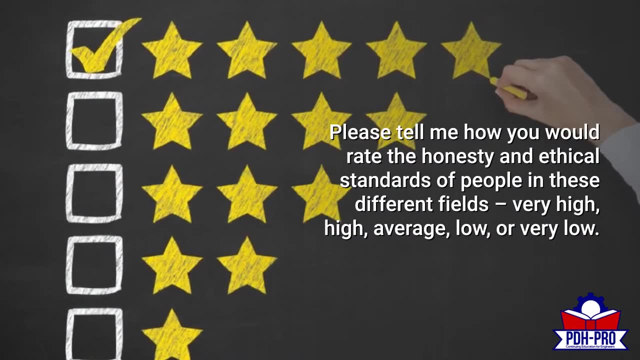 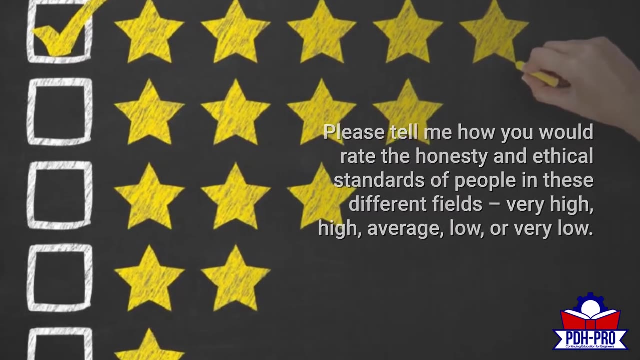 engineers had moved up to 65%. Gallup asked Americans this question. Please tell me how you would rate the honesty and ethical standards of people in these different fields – very high, high, average, low or very low. The Texas Board of Professional Engineers publishes all of its disciplinary decisions. 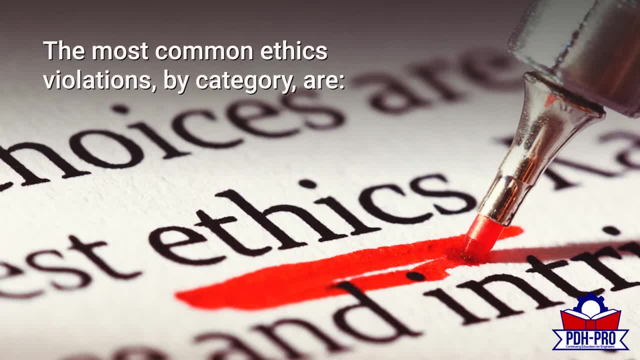 The most common ethics violations, by category, are: 1. Practicing without a license, 2. Negligence, 3. Improper use of seal and or title block, 4. Continuing education, 5. Felony conviction, 6. False statements. 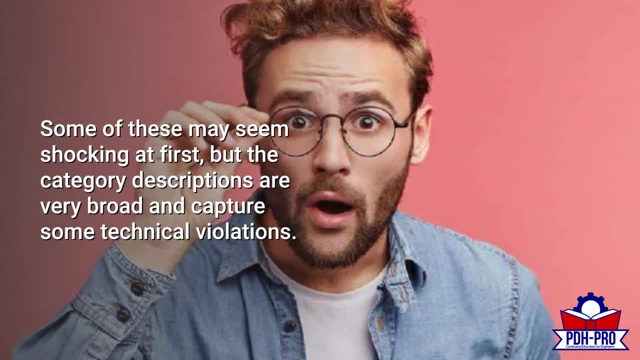 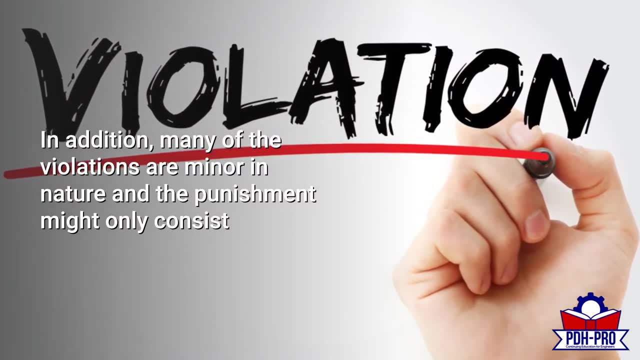 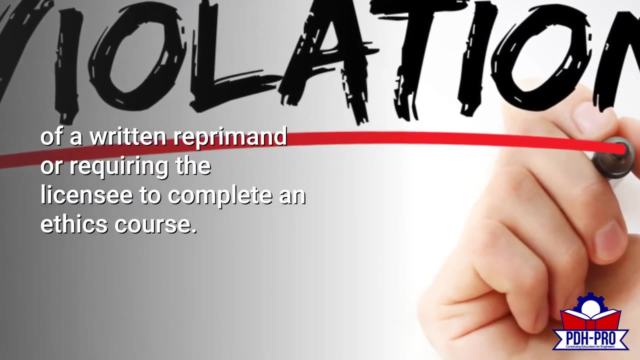 Some of these may seem shocking at first, but the category descriptions are very broad and capture some technical violations. In addition, many of the violations are minor in nature and the punishment might only consist of a written reprimand or requiring the licensee to complete an ethics course. Ethical behavior and professionalism is how 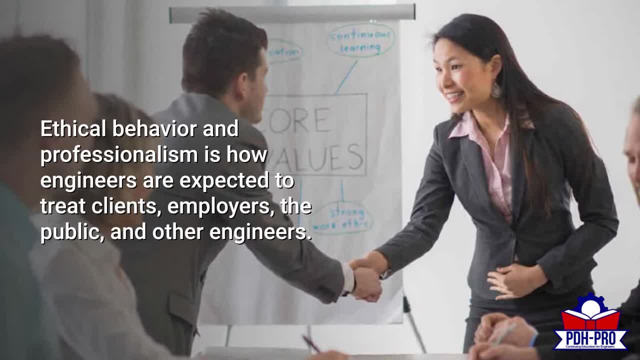 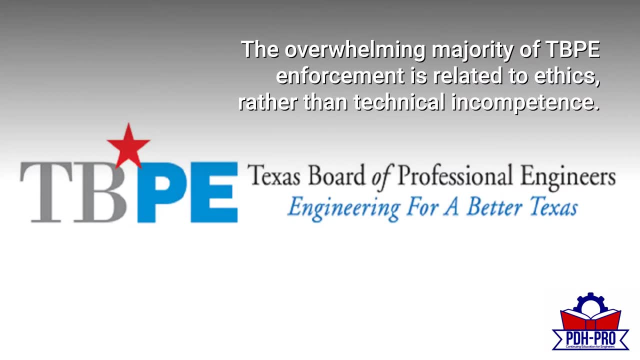 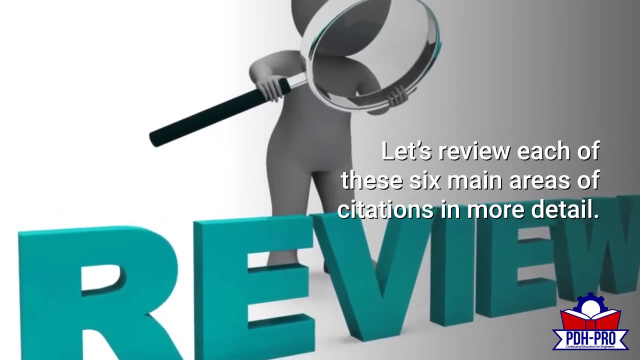 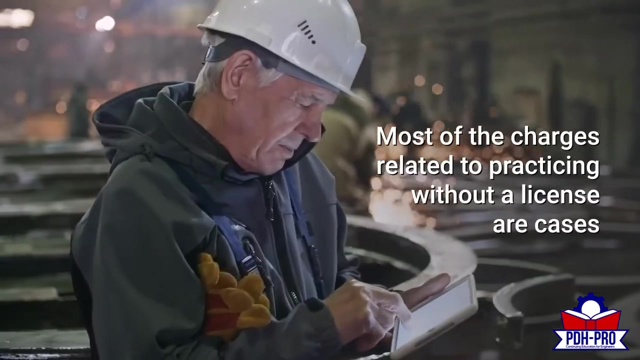 engineers are expected to treat clients, employers, the public and other engineers. The overwhelming majority of TBPE enforcement is related to ethics rather than technical incompetence. Let's review each of these six main areas of citations in more detail. 1. Practicing Without a License: Most of the charges related to practicing 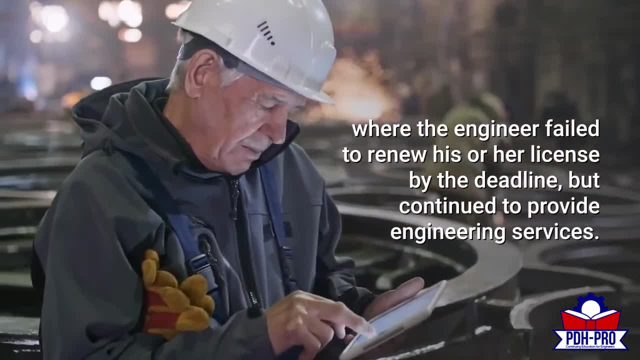 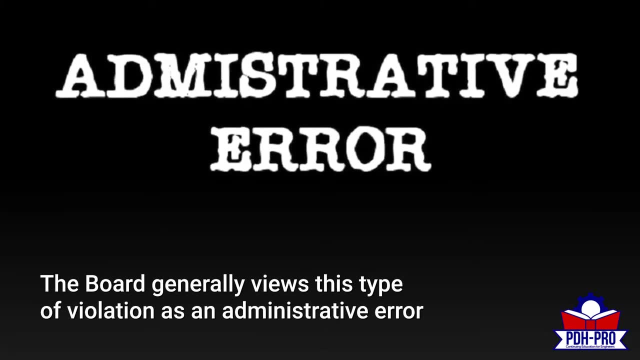 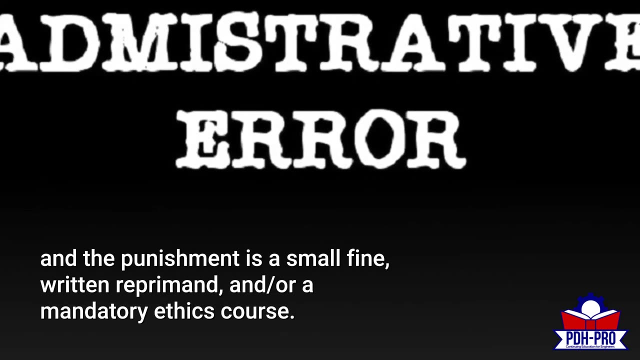 without a license are cases where the engineer failed to renew his or her license by the deadline but continued to provide engineering services. The Board generally views this type of violation as an administrative error and the punishment is a small fine written reprimand. 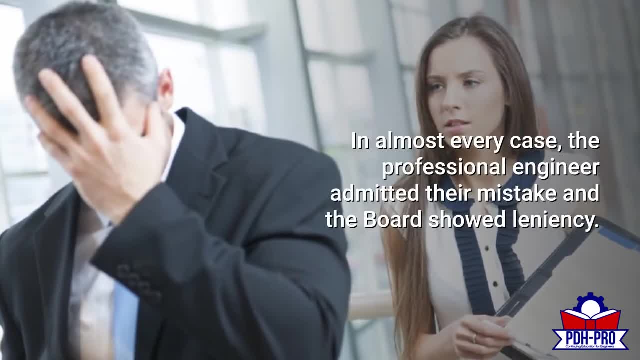 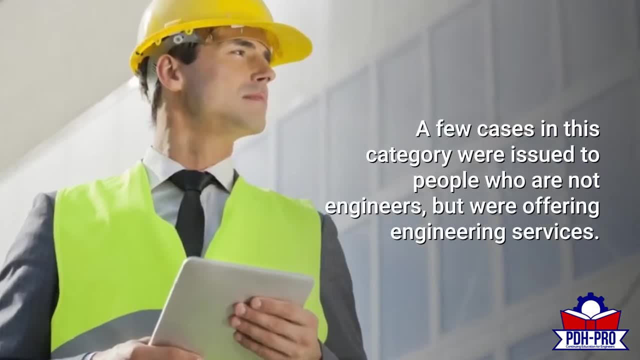 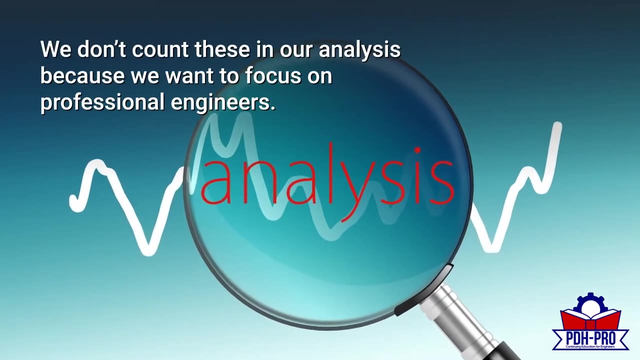 and or a mandatory ethics course. In almost every case, the professional engineer, The engineer admitted their mistake and the board showed leniency. A few cases in this category were issued to people who were not engineers but were offering engineering services. We don't count these in our analysis because we want to focus on professional engineers. 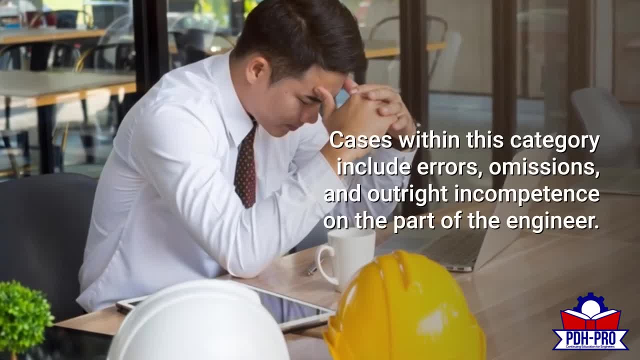 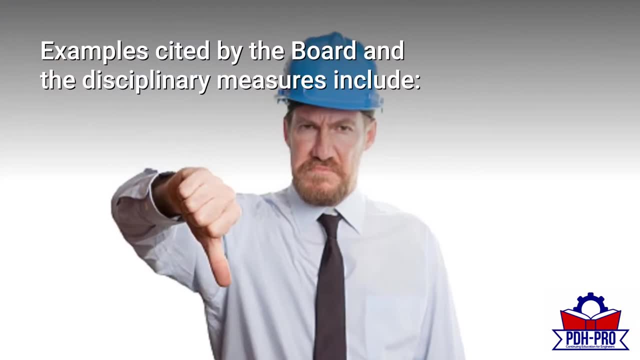 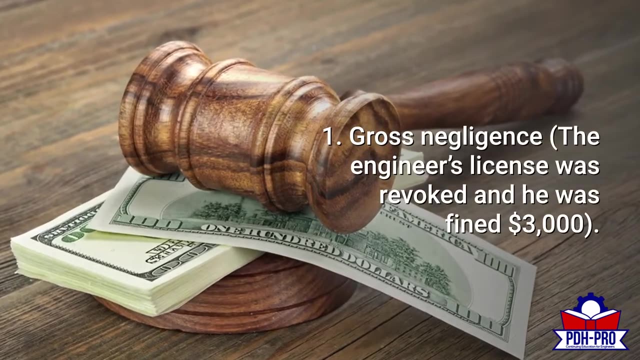 Violation 2 – Negligence. Cases within this category include errors, omissions and outright incompetence on the part of the engineer. Examples cited by the board and the disciplinary measures include: 1. Gross Negligence – The engineer's license was revoked and he was fined $3,000. 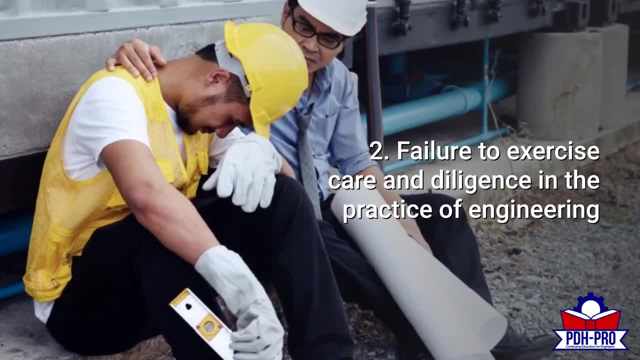 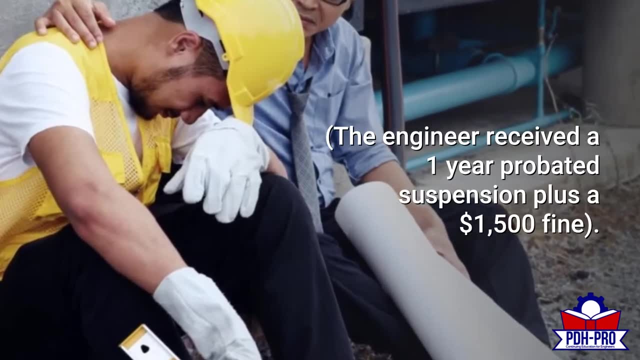 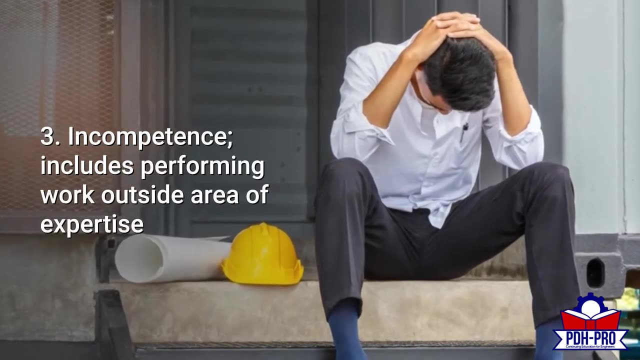 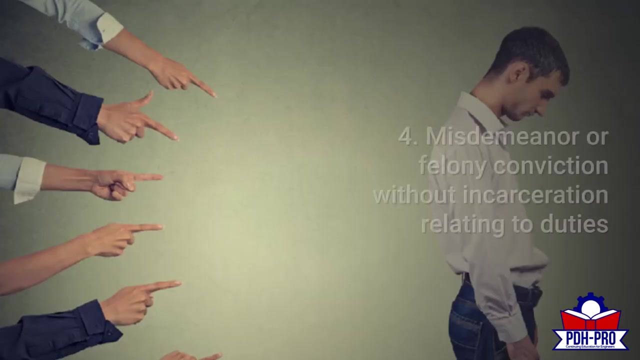 2. Failure to exercise care and diligence in the practice of engineering – The engineer received a one-year probated suspension plus a $1,500 fine. 3. Incompetence – Includes performing work outside area of expertise. The disciplinary decision included a three-year suspension and a fine of $3,000. 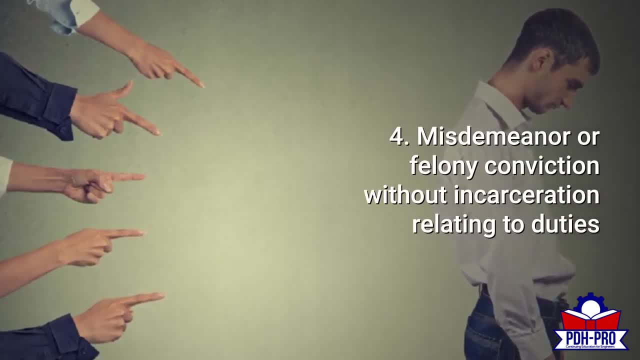 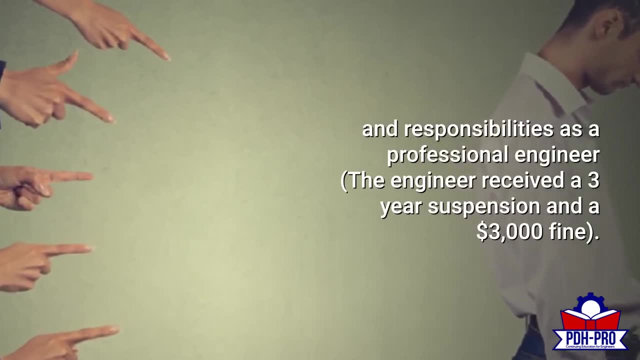 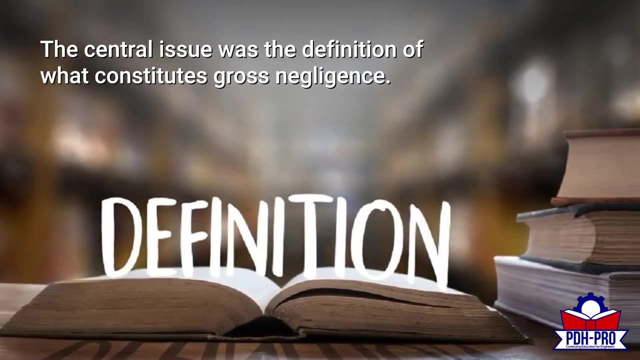 4. Misdemeanor or felony conviction without incarceration relating to duties and responsibilities as a professional engineer. – The engineer received a three-year suspension and a $3,000 fine. The central issue was the definition of what constitutes gross negligence – The general. 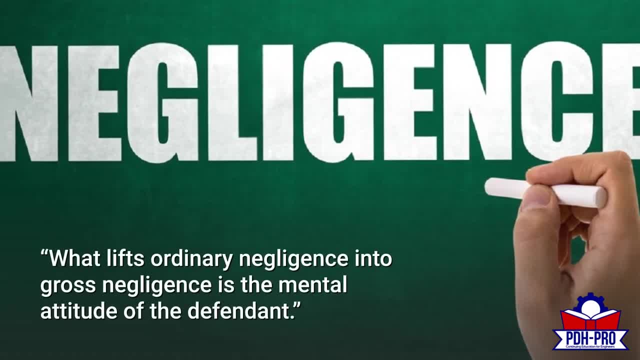 definition used by an engineer is gross negligence. The definition of gross negligence is gross negligence. The general definition used by an engineer is gross negligence. The general definition used by an engineer is gross negligence. The definition used by the digital engineering board is: – What lifts ordinary negligence? 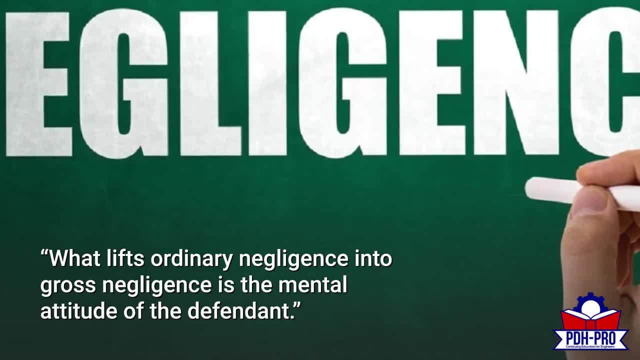 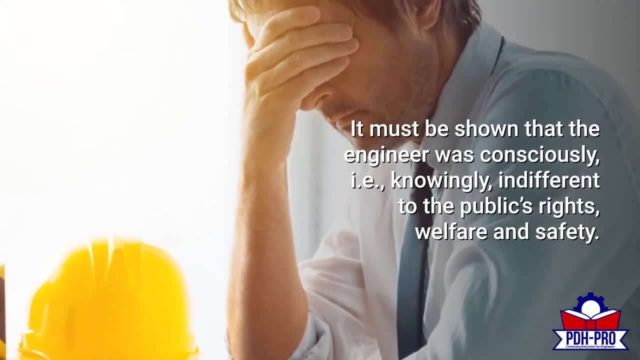 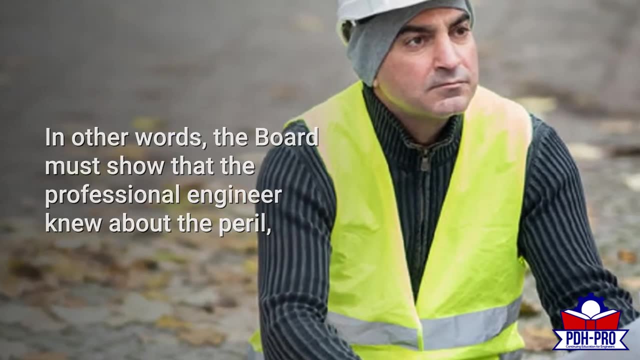 into gross negligence is the mental attitude of the defendant. It must be shown that the engineer was consciously indifferent to the public's rights, welfare and safety. In other words, the board must show that the professional engineer knew about the peril, but his acts or emotions demonstrated that he didn't care. 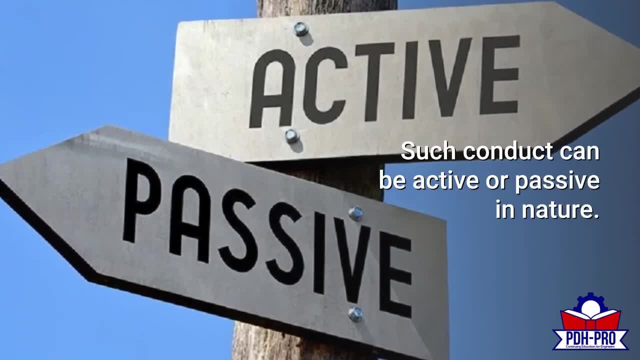 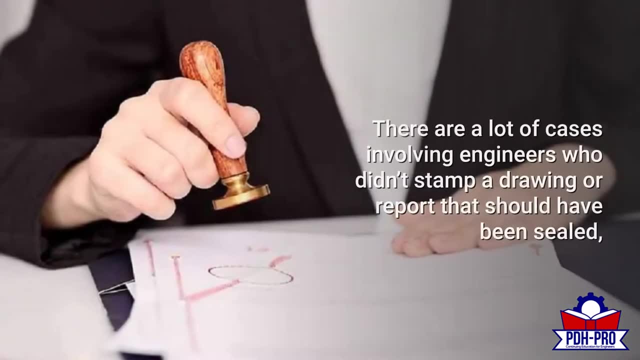 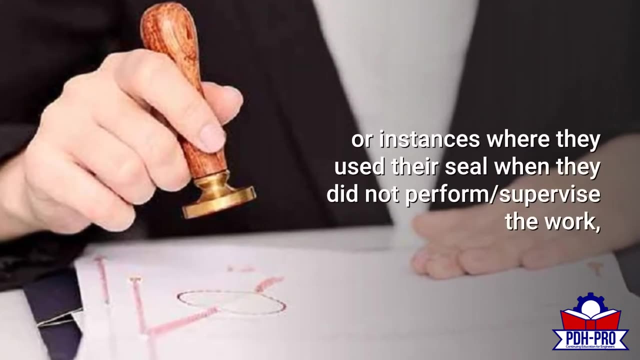 Such conduct can be active or passive in nature. Violation 3 – Improper use of seal and or title block. There are a lot of cases involving engineers who didn't stamp a drawing or report that should have been sealed, Or instances where they used their seal when they did not perform supervise the work. 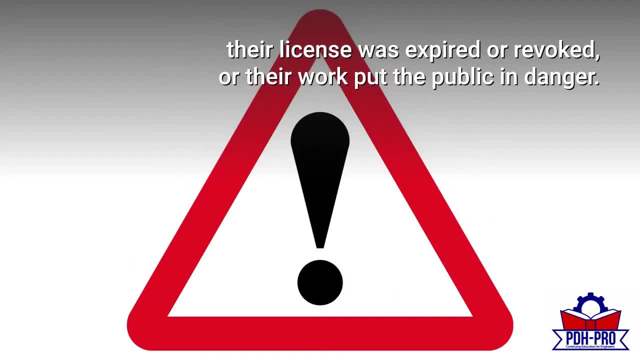 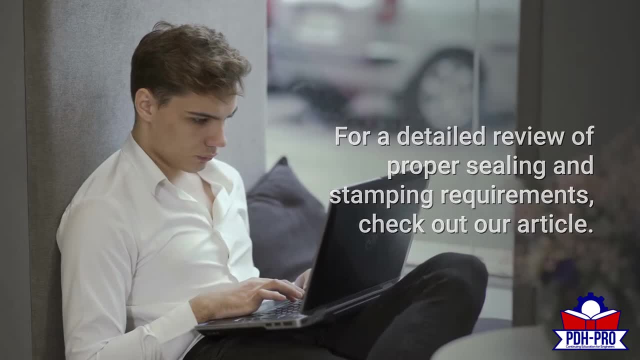 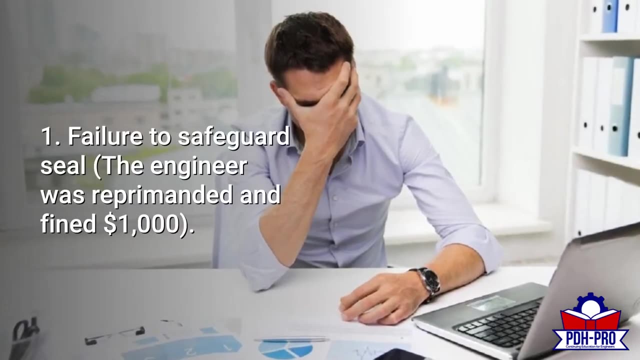 their license was expired or revoked or their work put the public in danger. For a detailed review of the proper sealing and stamping requirements, check out our article. Here are examples of citations with the penalties handed out by the board: 1.. 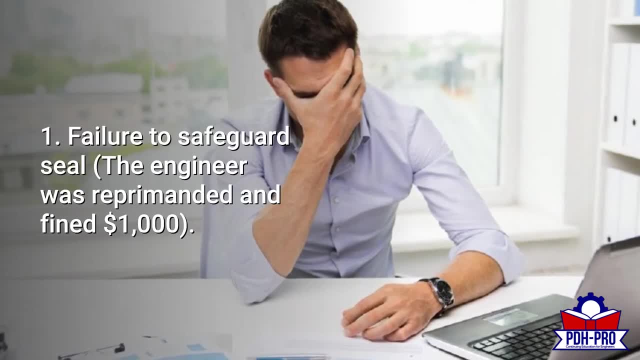 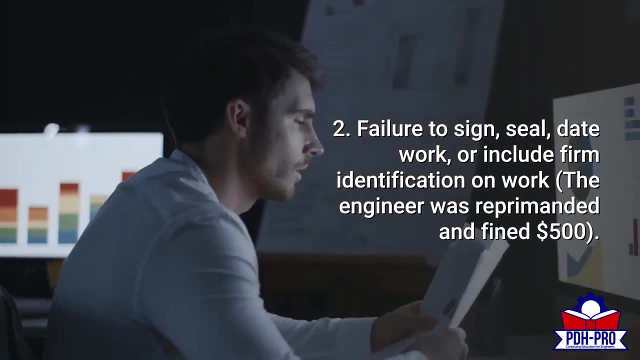 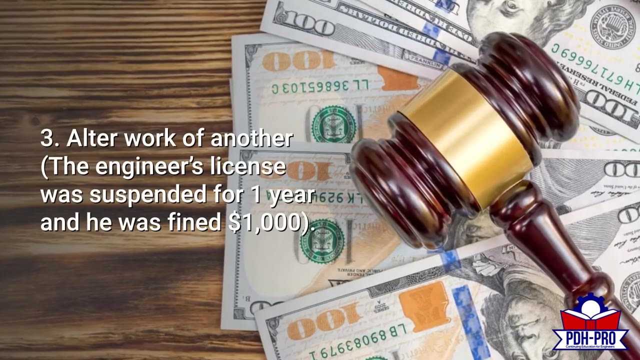 Failure to Safeguard Seal – The engineer was reprimanded and fined $1,000.. 2. Failure to Sign Seal Date Work or Include Firm Identification on Work – The engineer was reprimanded and fined $500.. 3.. 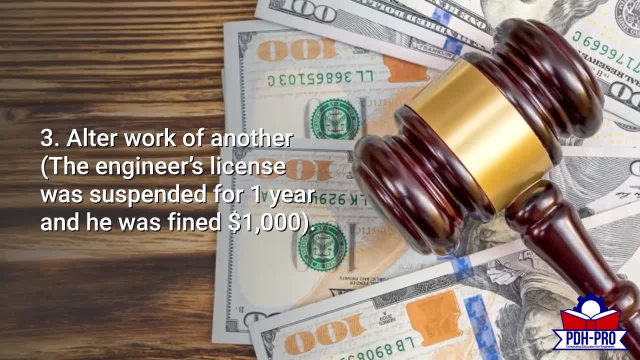 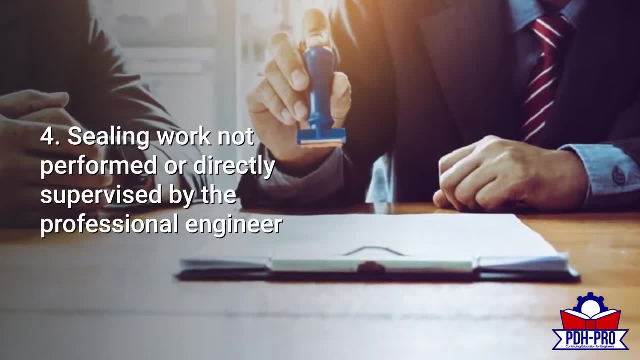 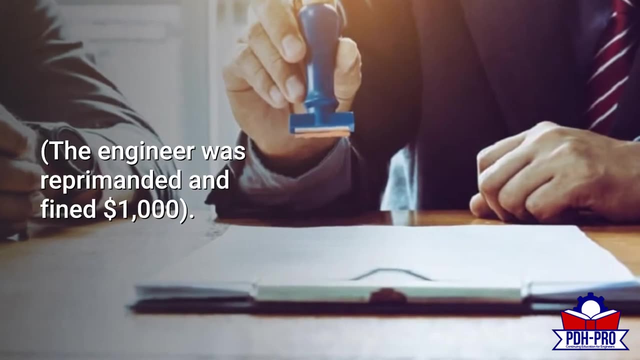 Alter Work of Another – The engineer's license was suspended for one year and he was fined $1,000.. 4. Sealing Work Not Performed or Directly Supervised by the Professional Engineer – The engineer was reprimanded and fined $1,000. 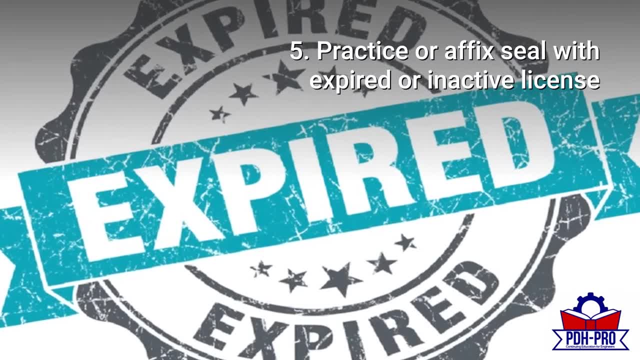 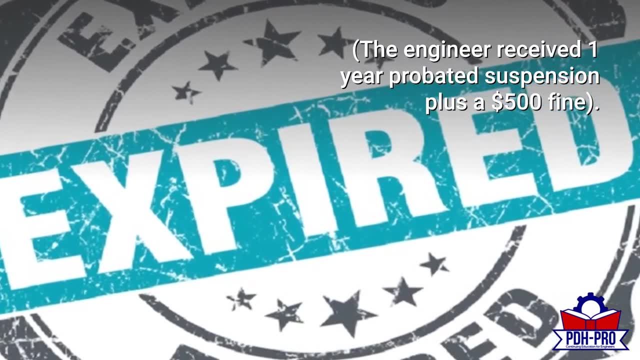 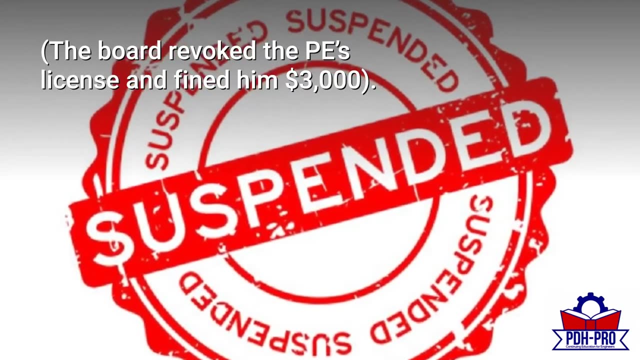 5. Practice or Affix Seal with Expired or Inactive License: – The engineer received one year probated suspension plus a $500 fine. 6. Practice or Affix Seal with Suspended License: – The board revoked the PE's license and. 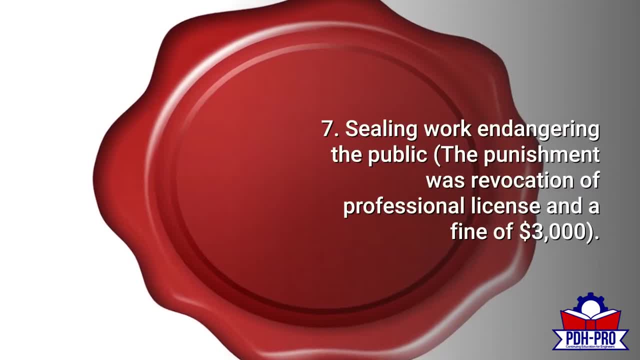 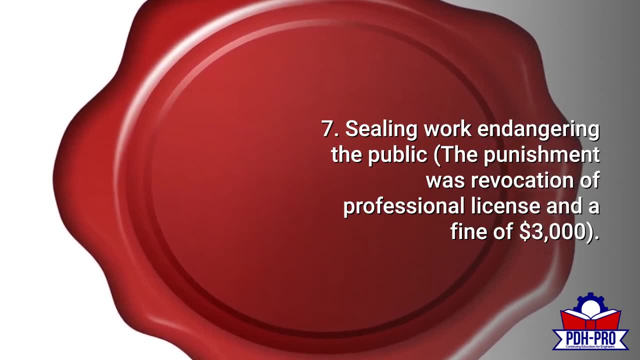 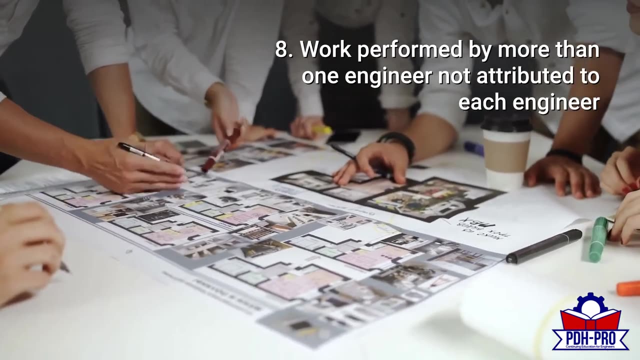 fined him $3,000.. 7. Sealing Work Endangering the Public – The punishment was revocation of professional license and a fine of $3,000.. 8. Work Performed by More Than One Engineer Not Attributed to Each Engineer – The board. 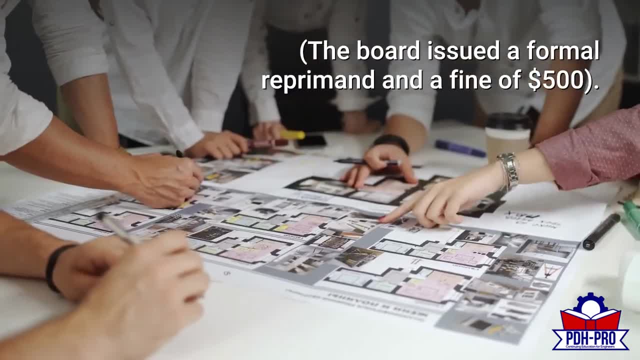 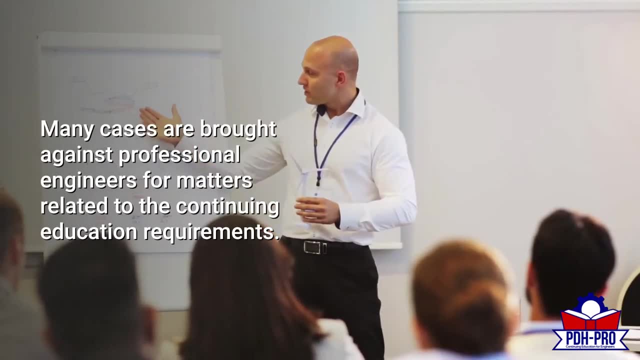 issued a formal reprimand and a fine of $3,000.. 9. clause a and a Off Edition. 7. Sealing Work Not Performed by we less than you. Many cases are brought against professional engineers for matters related to the continuing 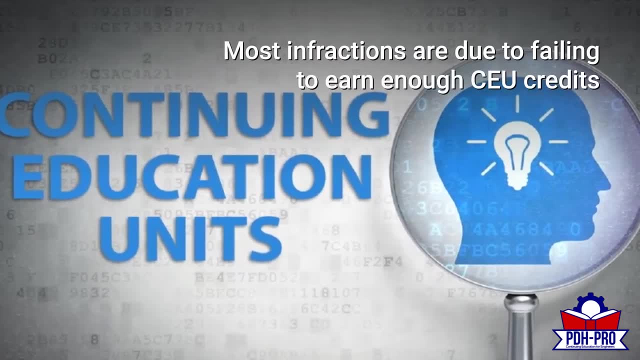 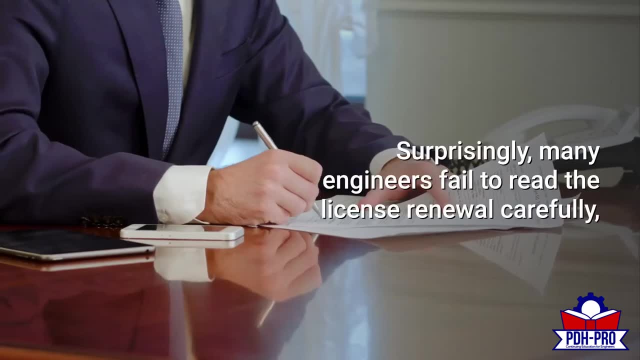 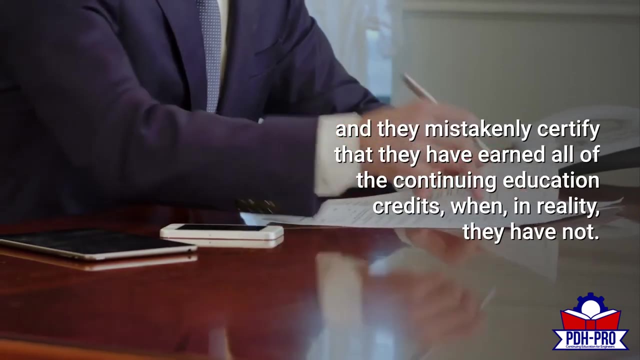 education requirements. Most infractions are due to failing to earn enough CEU credits or falsely reporting that all required hours were earned. Surprisingly, many engineers failed to read the license renewal carefully and they mistakenly certify that they have earned all of the continuing education credits. 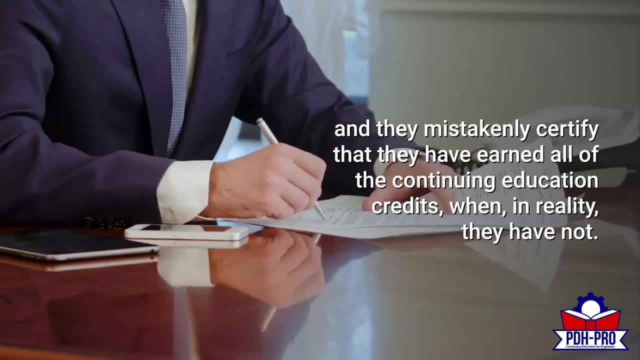 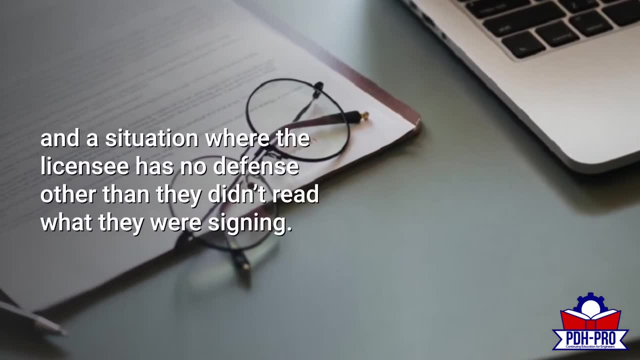 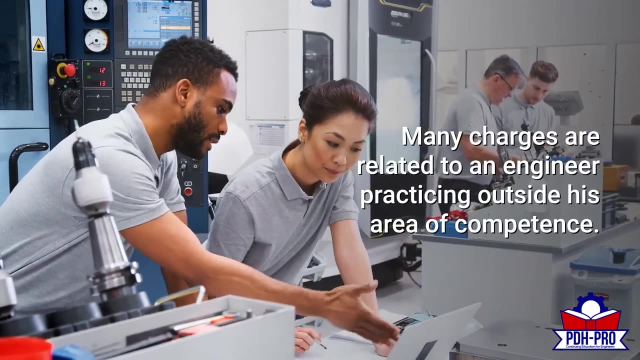 8. education credits when in reality they have not. This leads to a charge of making a false statement, which is clearly an ethics violation, and a situation where the licensee has no defense other than they didn't read what they were signing. Many charges are related to an engineer. 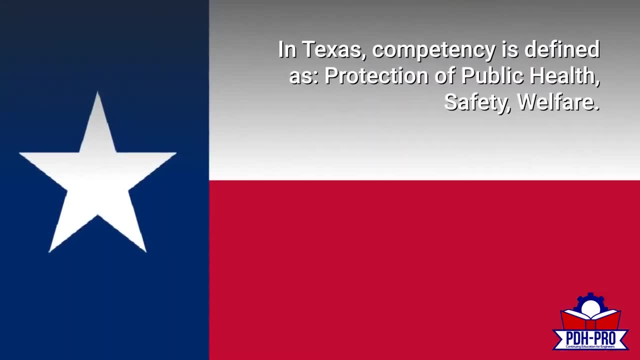 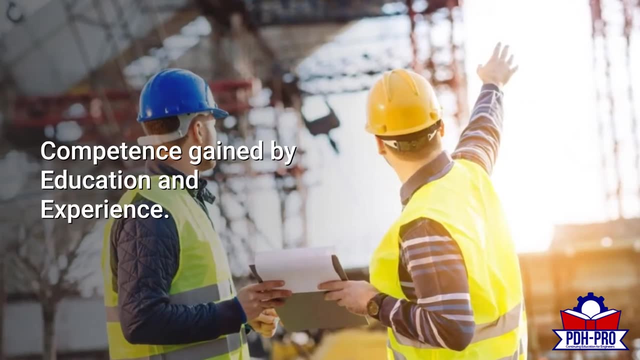 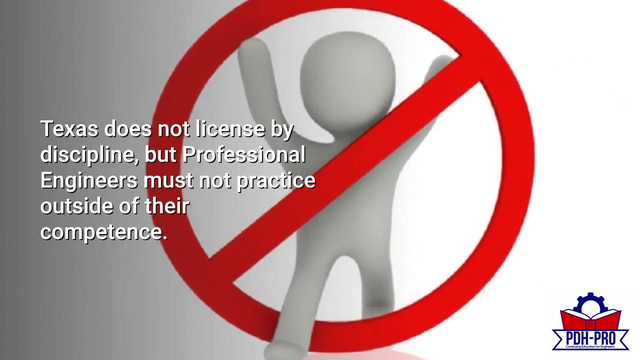 practicing outside his area of competence. In Texas competency is defined as protection of public health, safety, welfare, competence gained by education and experience. Texas does not license by discipline, but professional engineers must not practice outside of their competence. One thirty seven point five nine A. 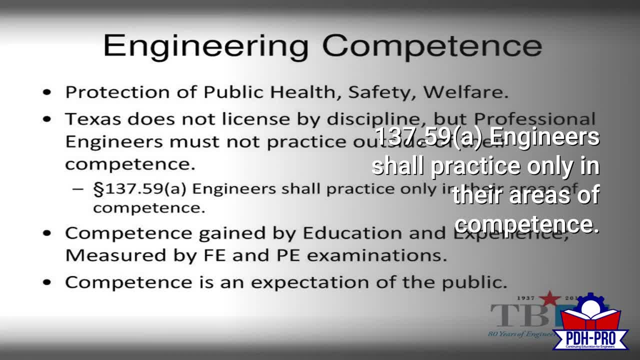 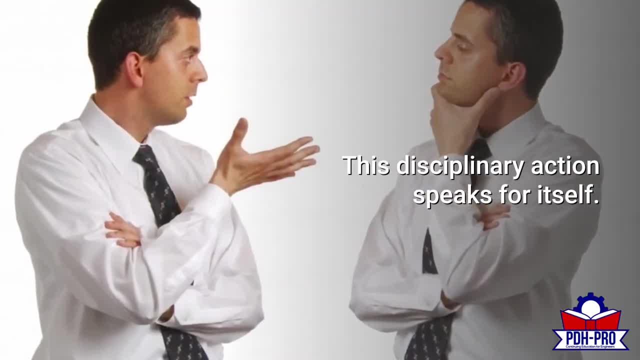 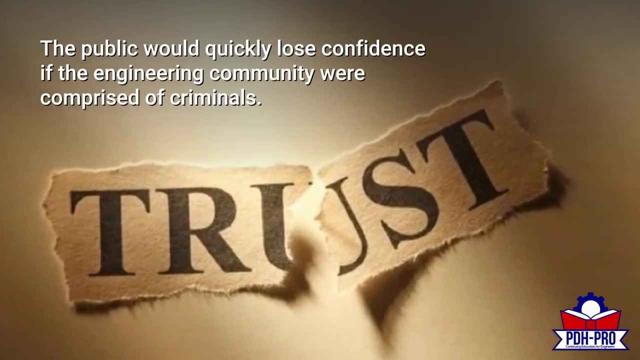 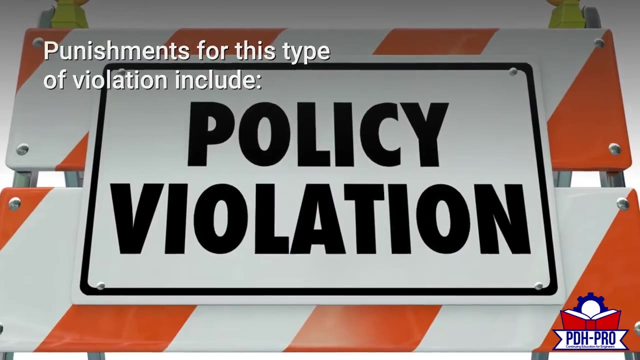 engineers shall practice only in their areas of competence. Violation: five felony conviction. this disciplinary action speaks for itself. Individual engineers are essentially ambassadors For the profession. the public would quickly lose confidence if the engineering community were comprised of criminals. Punishments for this type of violation include one misdemeanor or felony. 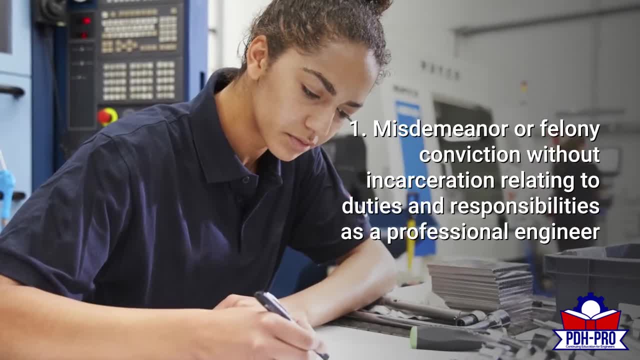 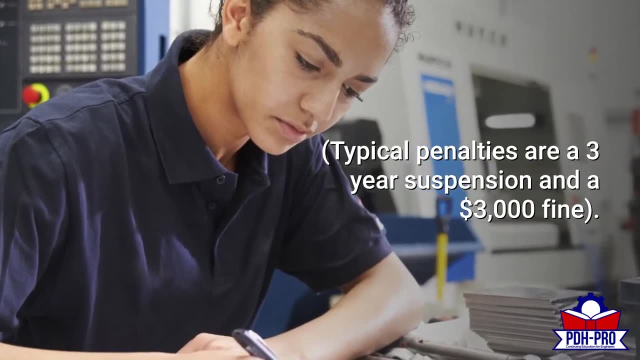 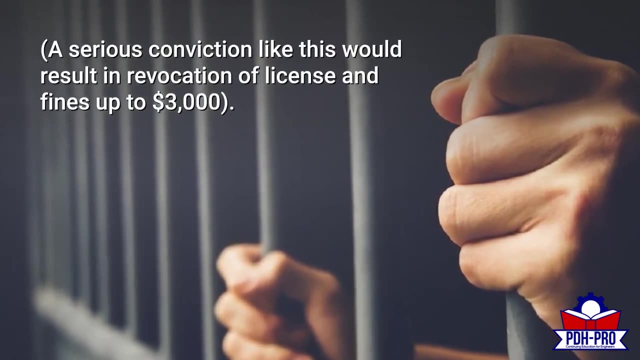 conviction without incarceration relating to duties and responsibilities As a professional engineer. typical penalties are a three year suspension and a three thousand dollar fine to felony conviction. with incarceration a serious conviction, This would result in revocation of license and fines up to three thousand dollars. 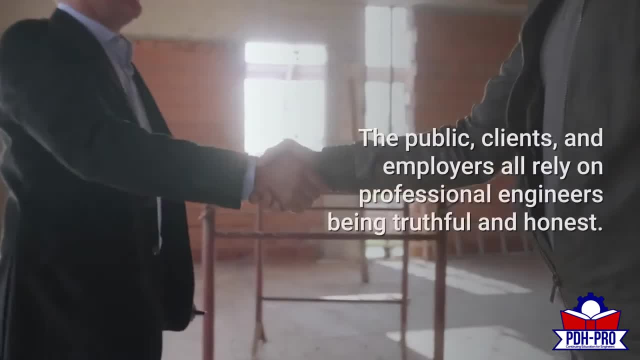 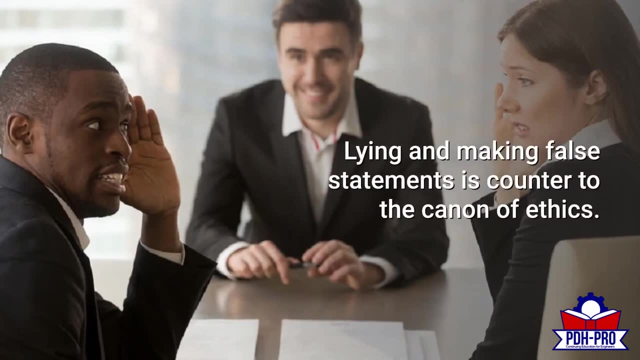 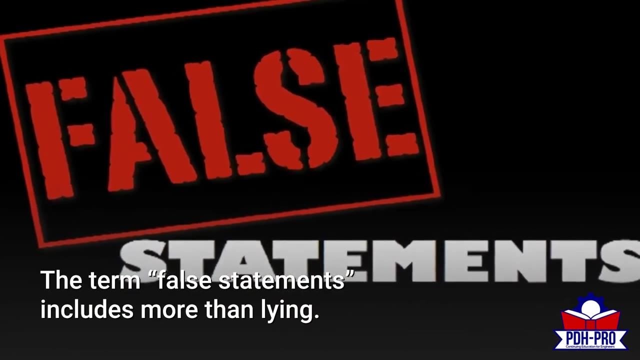 Violation: six false statements. The public, clients and employers all rely on professional engineers being truthful and honest. lying and making false statements is counter to the canon of ethics. The term false statements includes more than lying. It can include deceptive business practices, false advertising and not 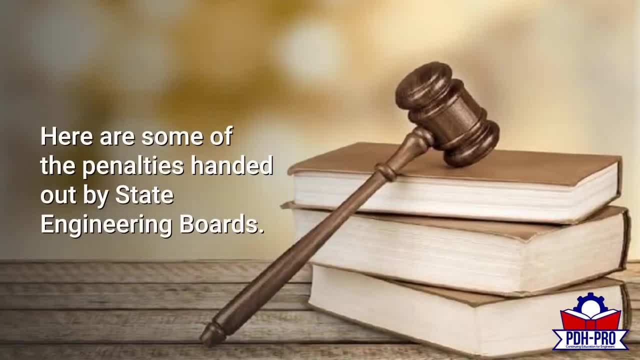 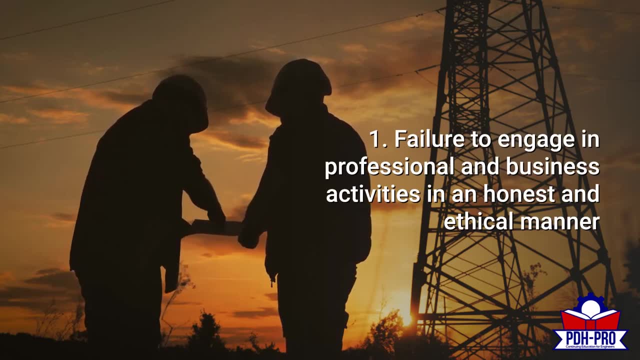 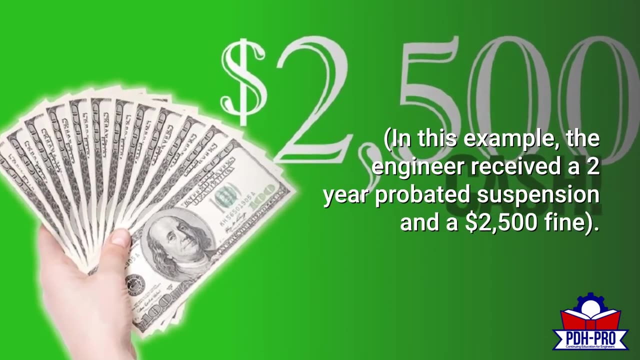 using conflicts of interest to clients or employers. Here are some of the penalties handed out by state engineering boards: One: failure to engage in professional and business activities in an honest and ethical manner. In this example, the engineer received a two year probated suspension and a twenty five hundred dollar fine. 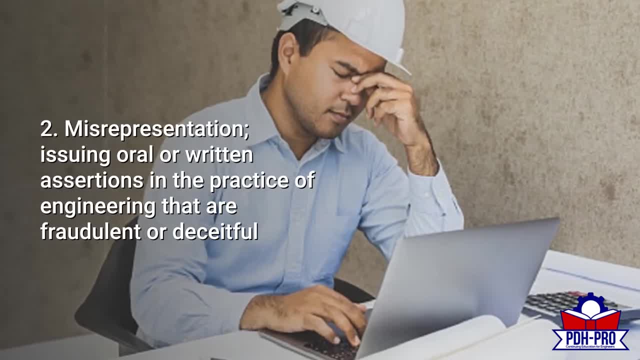 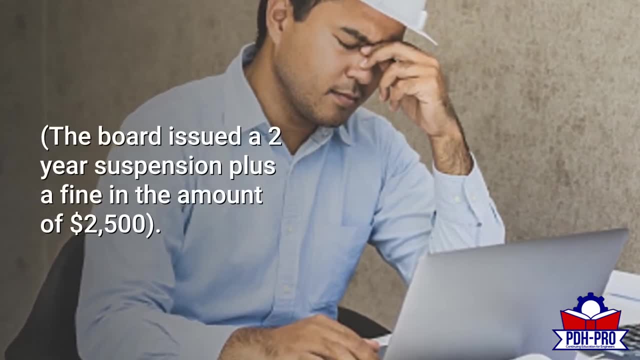 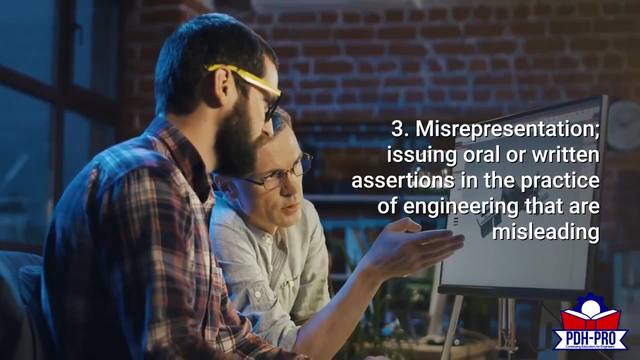 Two: misrepresentation: issuing oral or written assertions in the practice of engineering that are fraudulent or deceitful. The board issued a two year suspension plus a fine in the amount of twenty five hundred dollars. Three: misrepresentation: issuing oral or written assertions in the practice of engineering that are misleading. 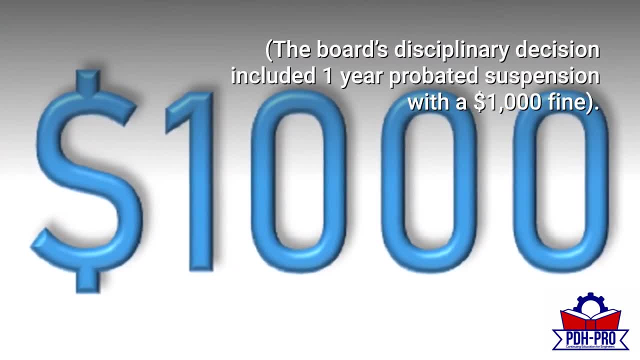 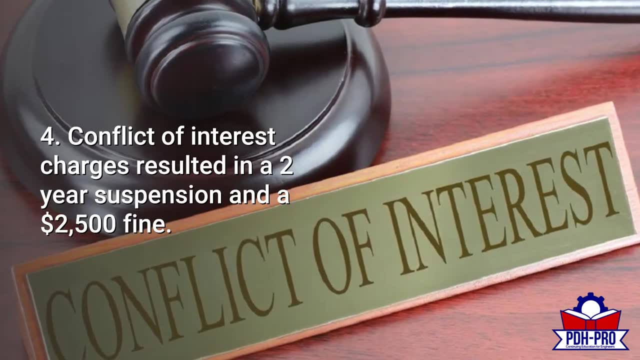 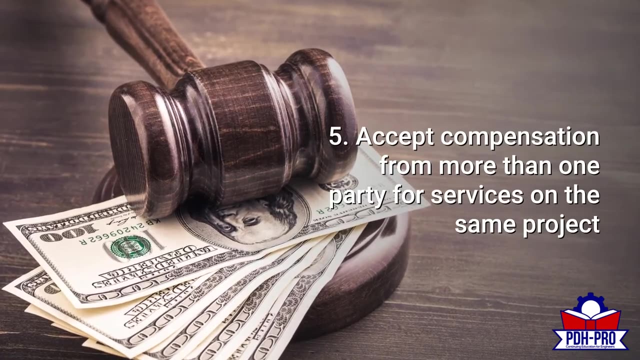 The board's disciplinary decision included one year probated suspension with a one thousand dollar fine. Four conflict of interest charges resulted in a two year suspension and a twenty five hundred dollar fine. Five: accept compensation from more than one party for services on the same project. 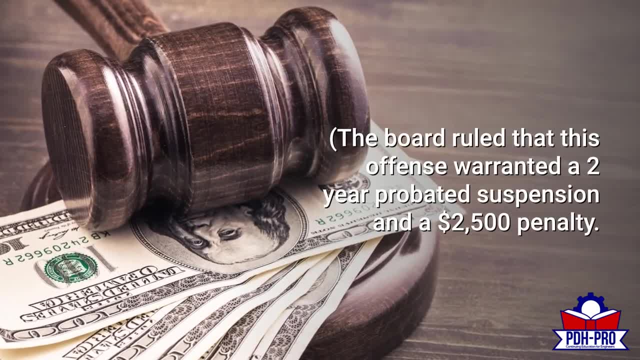 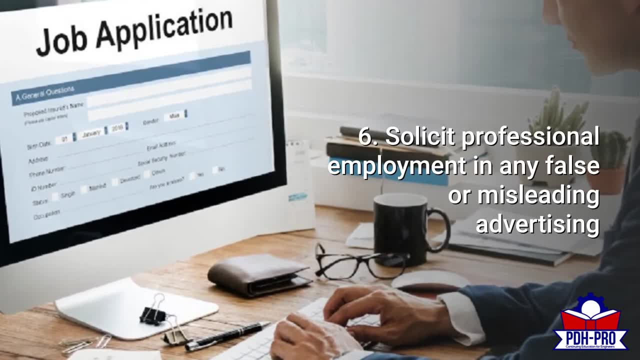 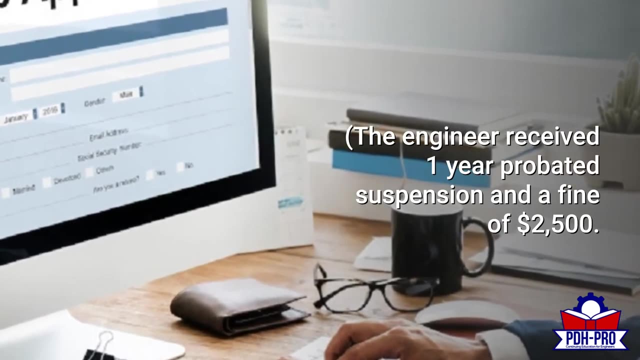 The board ruled that this offense warranted a two year probated suspension and a twenty five hundred dollar penalty. Six solicit professional employment in any false or misleading advertising. The engineer received one year probated suspension and a fine of twenty five hundred dollars. What can you do if an engineering board 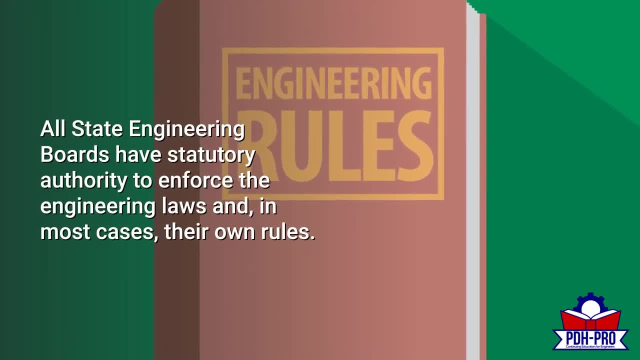 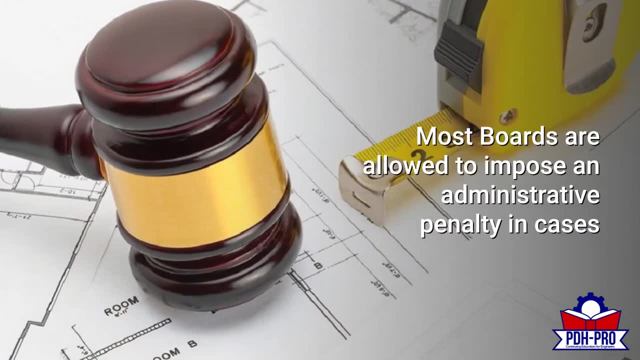 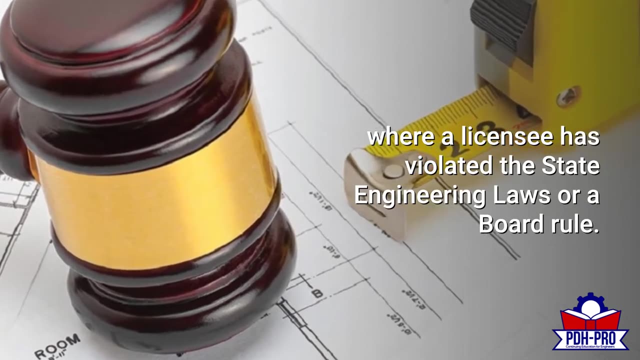 sanctions you All. state engineering boards have statutory authority to enforce the engineering laws and, in most cases, their own rules. Most boards are allowed to impose an administrative penalty in cases where a licensee has violated the state engineering laws or a board rule. the state engineering board may suspend. 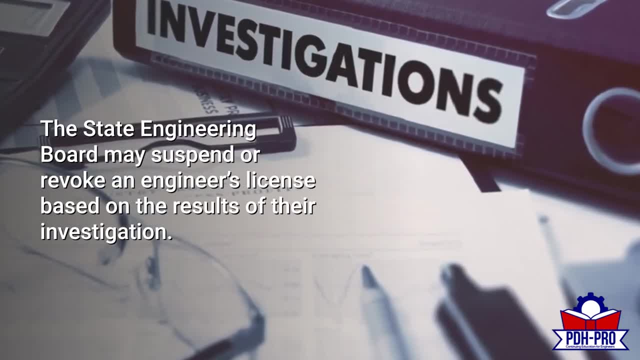 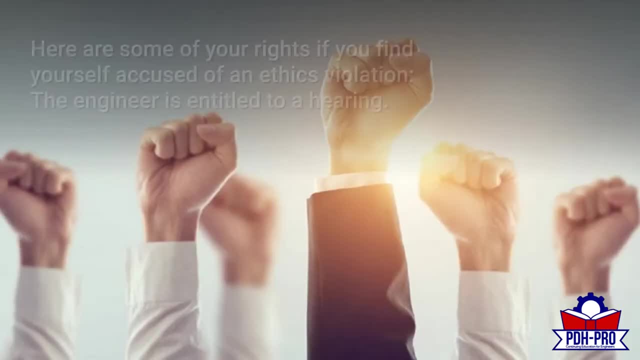 or revoke an engineer's license based on the results of their investigation. If this happens, that person has rights, Just as a person who is charged with a crime does. Here are some of your rights If you find yourself accused of an ethics violation. 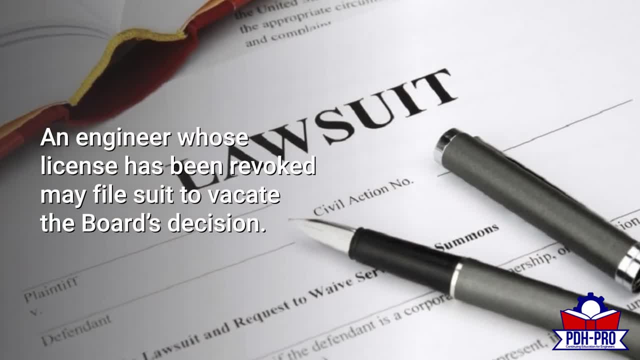 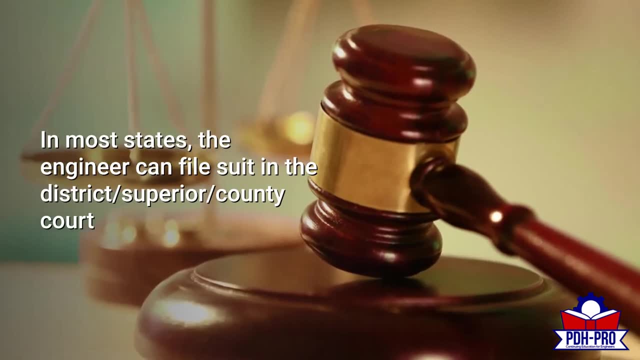 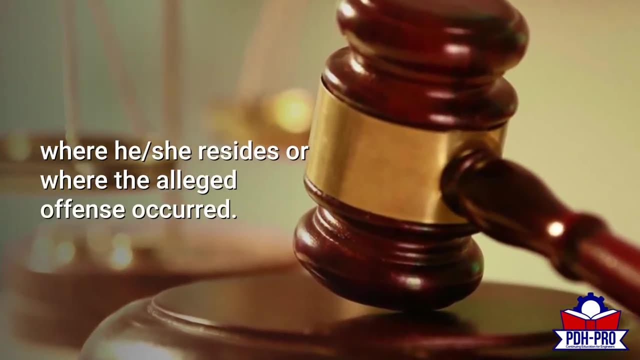 the engineer is entitled to a hearing. An engineer whose license has been revoked may file suit to vacate the board's decision. In most states, the engineer can file suit in the district superior county court where he, she resides or where the alleged offense occurred. 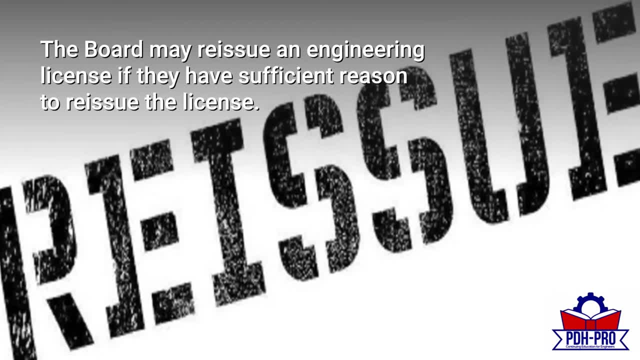 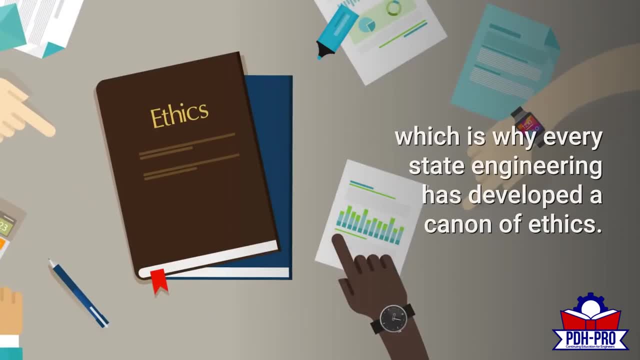 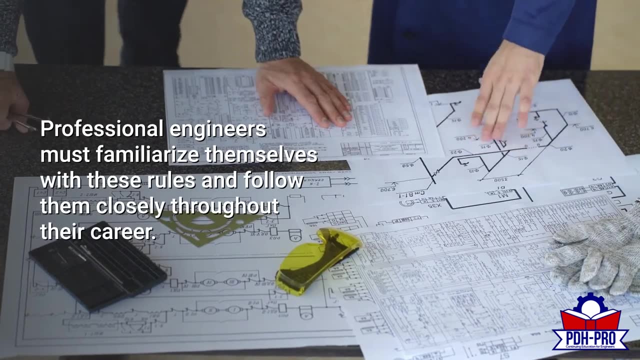 The board may reissue an engineering license If they have sufficient reason to reissue the license. Engineering ethics is a critical part of the work that engineers do, which is why every state engineering board has developed a canon of ethics Professional engineers must familiarize. 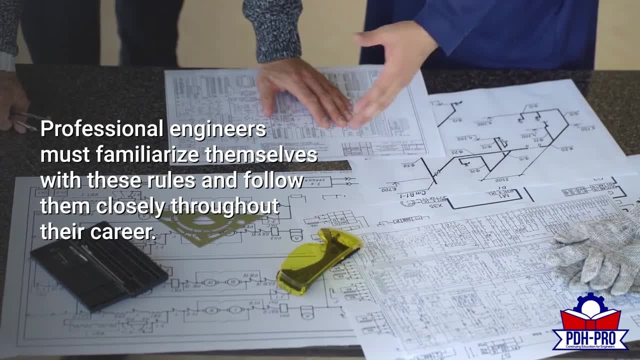 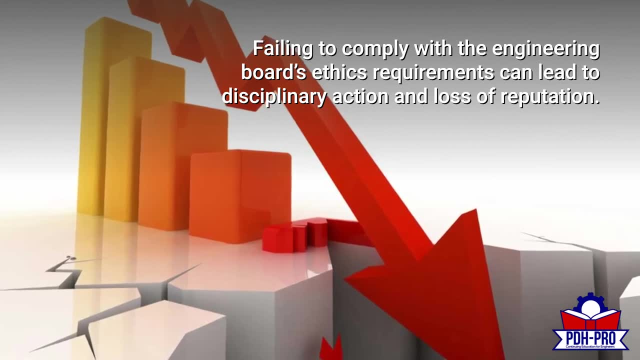 themselves with these rules and follow them closely throughout their career. Failing to comply with the engineering board's ethics requirements can lead to disciplinary action and loss of reputation. The good news is, it's easy to know how to conduct your self in a professional capacity.